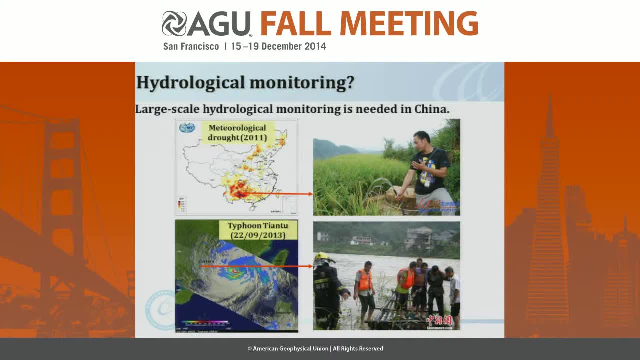 So, even though at the center of the drought there's still the soil, moisture is high and the people can take the stream flow for irrigation, So the crop land can sustain during the drought, And also for the climate system. monitoring system can capture this kind of typhoon even very well. 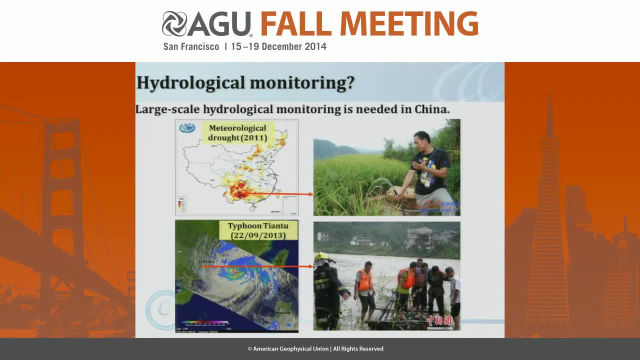 and we can see. We can see this kind of typhoon is coming. However, if we look close, for only a very limited area, we do have this flooding risk. So that's the difference between the hydrological monitoring and the climate monitoring. 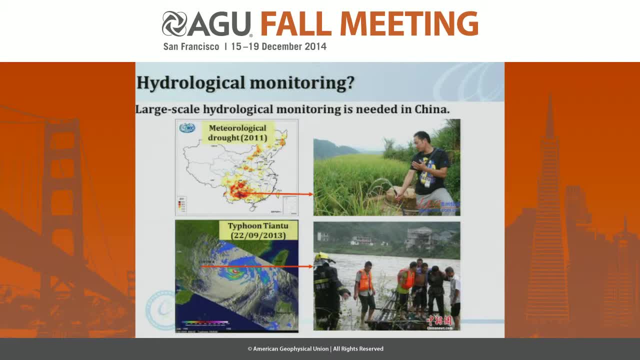 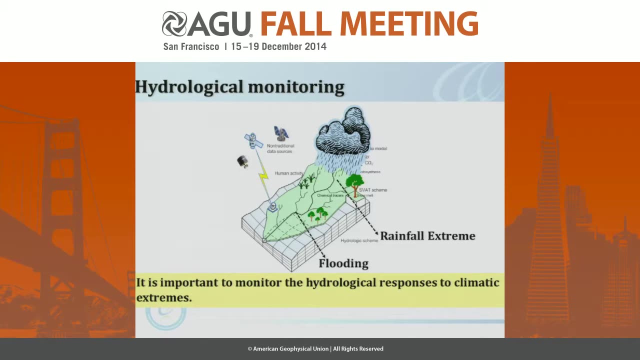 Climate monitoring. it can give a large scale change. However, the ground details- it usually is not covered with the ground details. So we need to build a hydrological monitoring system. We have to build a hydrological monitoring system for China. This shows how the model can work. 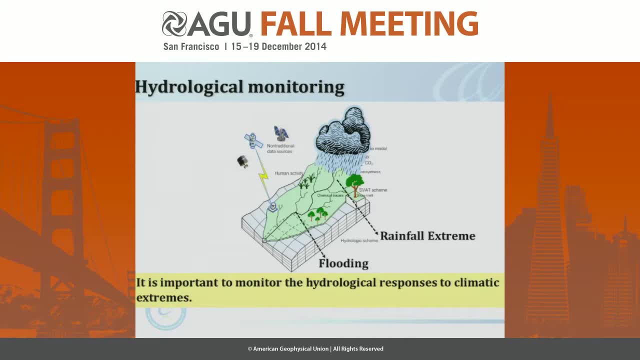 If there is a rainfall extreme, the location of the rainfall extreme actually may not be the same as the location of the hydrological extreme. We all know the decasement can accumulate the rainfall into the railway, So there will be a gap between this kind of meteorological extreme and the hydrological extreme. 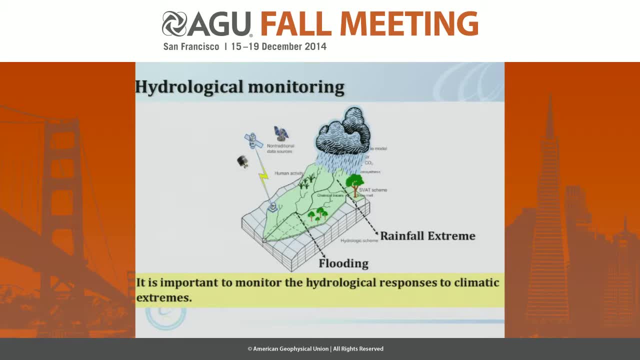 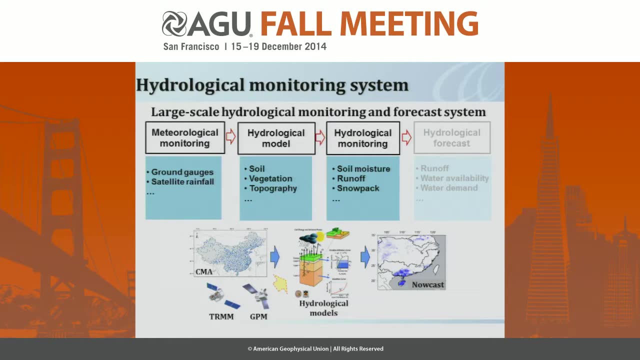 So that's the difference: hydrogen stream. So we need a model to build the connection between them. We have developed a large-scale hydrogen monitoring and forecast system for China. Here's the basic logic: We take the meteorological monitoring data from the climate monitoring system and put it into the hydrogen models and run the model. 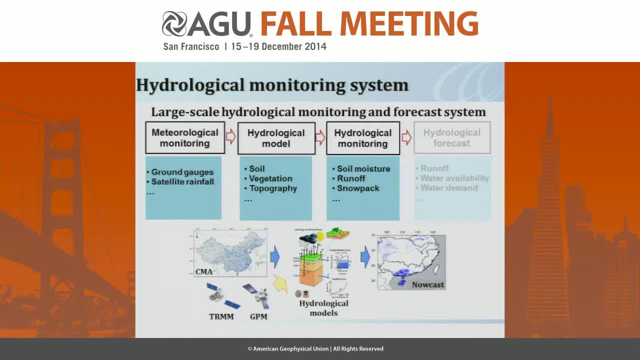 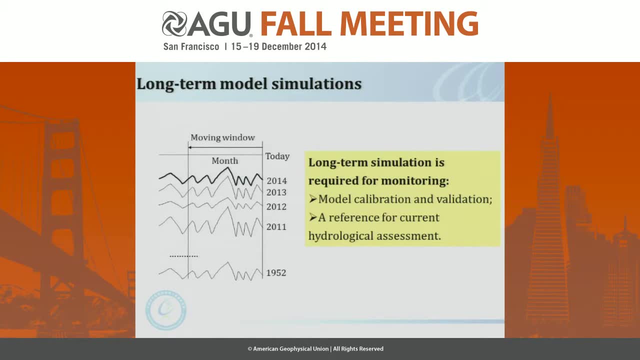 to get the hydrogen monitoring. So we'll get the initial condition for future forecast. But before I talk more detail about the near real-time monitoring, I think we need to have a long-term model simulation first. Why we need this? Because our target is for the near real-time monitoring. but why we need a 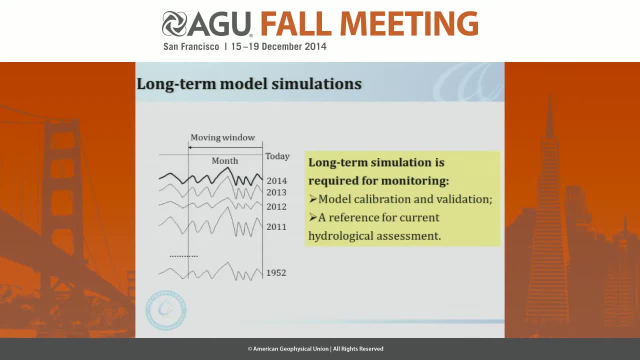 long-term model simulation. There are two reasons for that. One is we use the model. we need to make sure the model can work well in this region, So we need a long-term simulation for model calibration and the validation. Another reason is we need a reference for the current assessment When we say this. 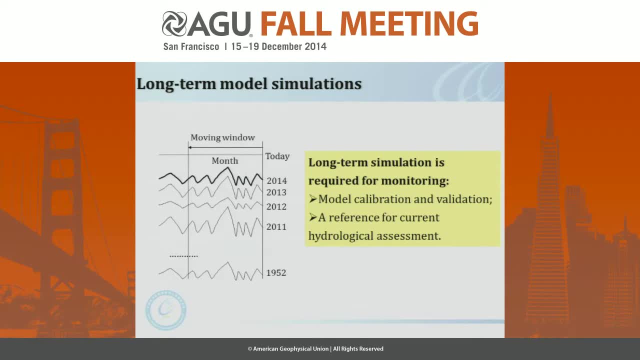 region has a risk of flooding or drought. we can decide to determinate this from the absolute values of discharge or stream flow. Actually, what we do is compare the current state to the historical data. Then if this data is consistent, then we can determine if the current state is extremely high in. 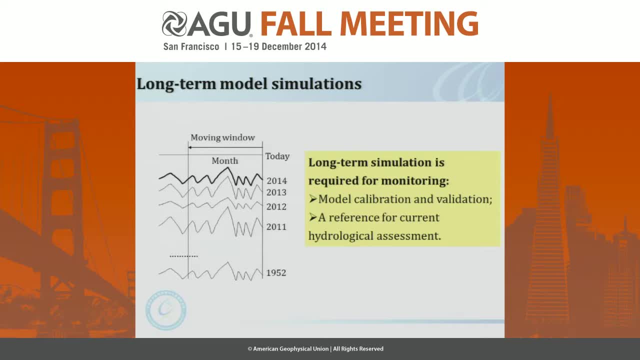 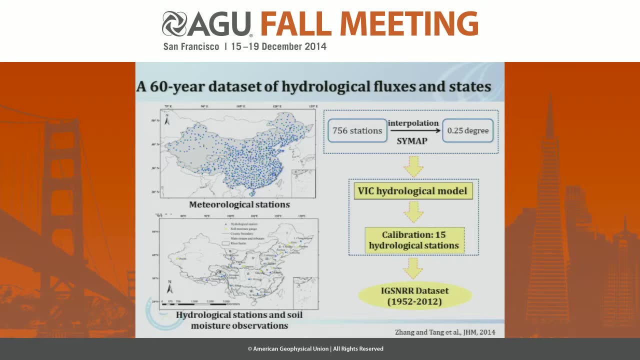 the past several decades, or extremely dry in the past decades. So, firstly, we produced a 30-year status of hydrologic flux in the states in China. What we do is we get the meteorological forcing from Chinese meteorological administration, We interpret the data into a quarter degree and we put 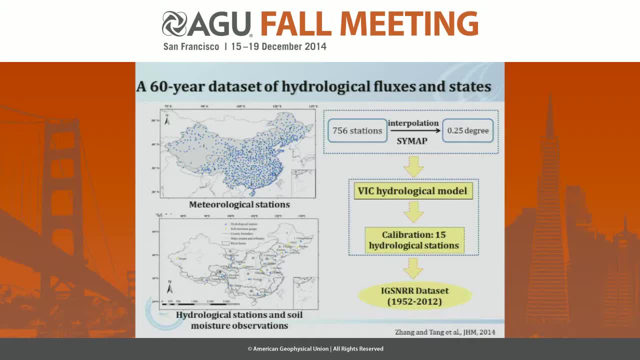 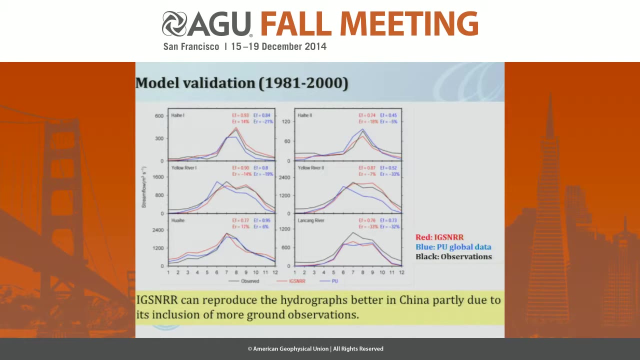 the forcing into the wake hydrological model And we carefully calibrate the model against the hydrological observations So we gather this kind of long-term data set that we call the IGS-NR data set. We validate this model in a 20-year period when 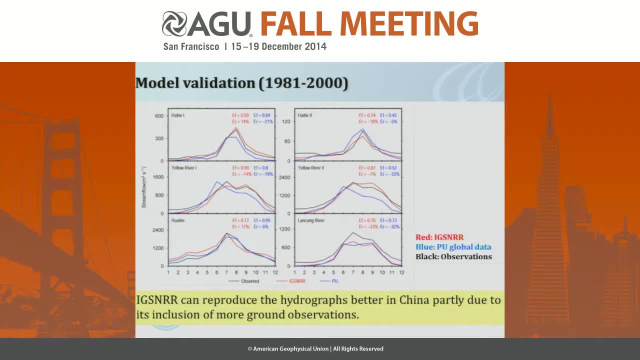 we have the ground observations. This will compare the IGS-NR stream flow with the global data set from Princeton University. So we can see the black line shows the observation and the blue one shows the estimate from Princeton University and the other line shows our estimate. It is not surprising: our data performs well in 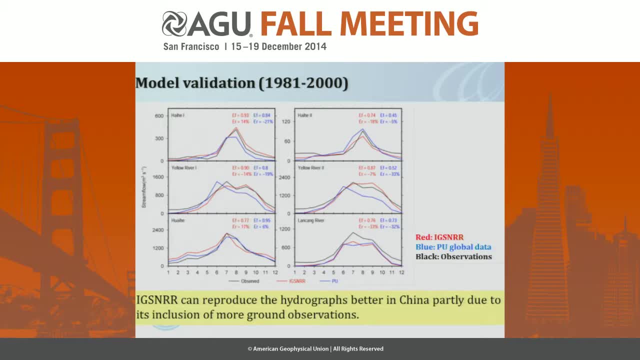 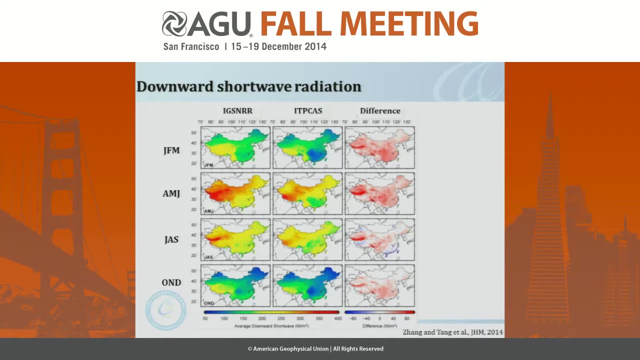 China because we use more ground observations in China. We also evaluate the downward shortwave radiation. The left column shows the estimate from our model and the center column shows a data set from ITP, Chinese Academy of Science, The ITP data set. they use much more ground shortwave. 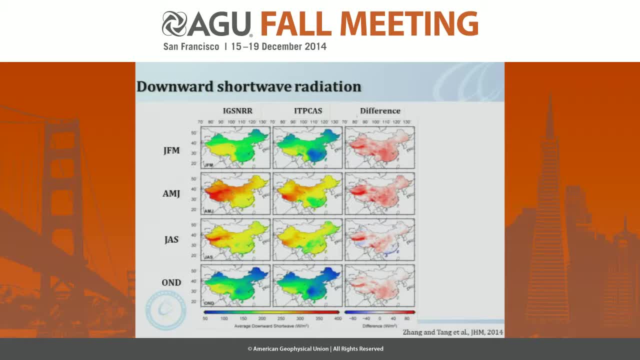 radiation observation and combined with the remote sensing data. So we knew that data will have better estimate over shortwave radiation. So we compare them and the difference actually is small. shows that our model can well capture the. they produce the shortwave radiation. What do we? in winter get some big difference. However, in summer, in the 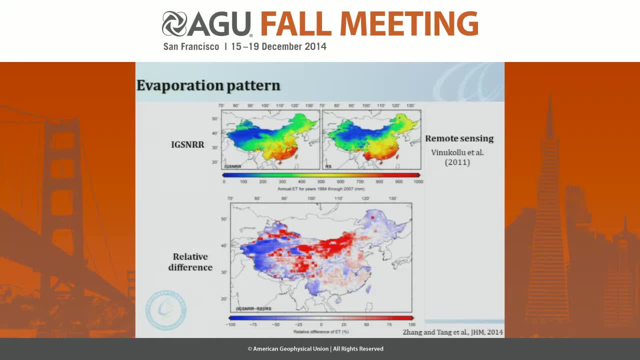 season we really care about. the difference is small And we're also assessing the opulation pattern and compare the opium transpilation pattern with the remote sensing and based estimate from Princeton University. Actually the pattern agree with each other very well. but if we 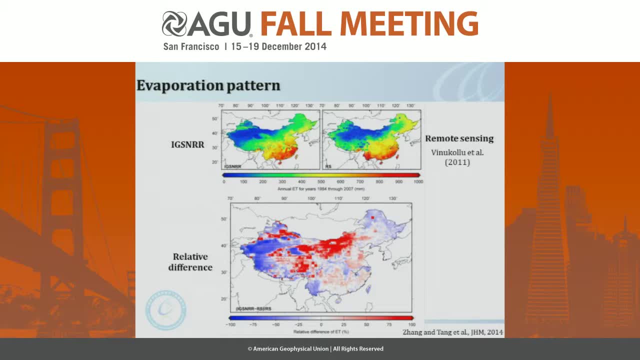 calculate the relative difference. the lanz curism is small in the Eastern China. however, it is not in the West. There's two reasons. One reason is in Western China the European nation is small. so when we calculate the relative difference, there is 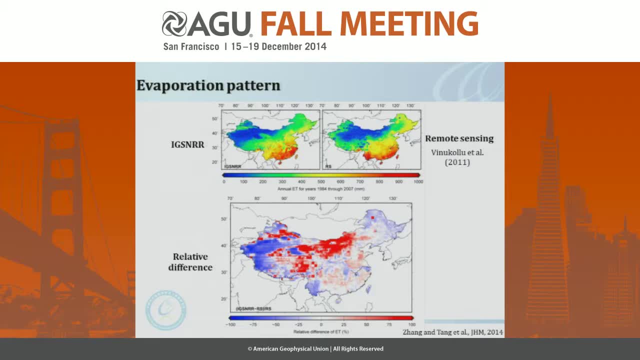 usually a small difference, make it's a larger negative difference. Another reason is: in West China every nation has to use a relative difference because theич And now the reason is in each other: A big difference and a relative difference, The. I chance that they have relative. 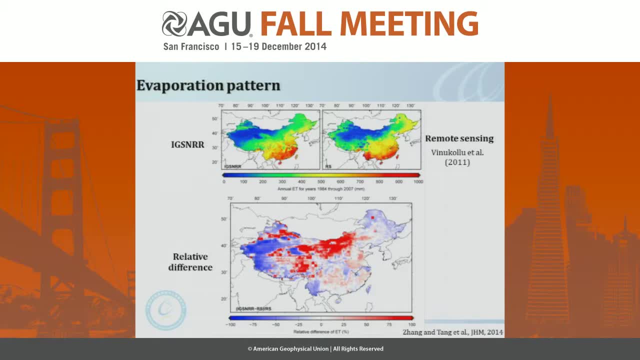 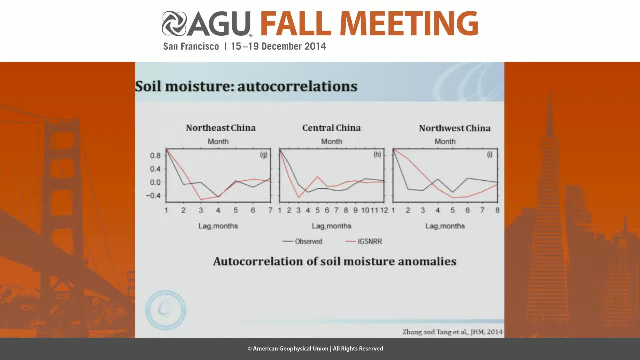 Another reason is in Western China we don't have much ground observations, so the data quantity may be a problem in that side. We also assessed the soil moisture. We cannot compare the soil moisture at the station directly, so we compared the autocorrelations. 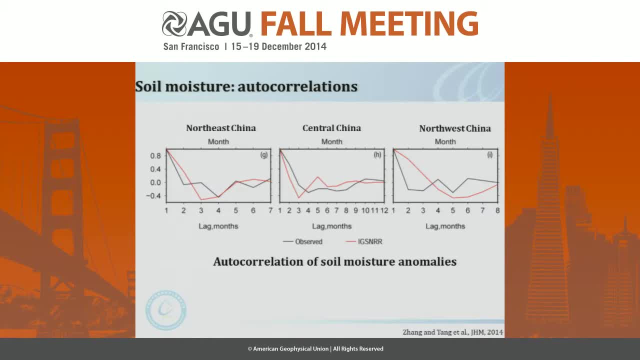 of soil moisture. It shows the memory of the soil moisture, The model estimate with observation in Eastern China and Central China. However, in Northwest China, the model shows the long memory. however, the observation shows much shorter memory. I think this is also the problem because we don't have much observation in the West China. 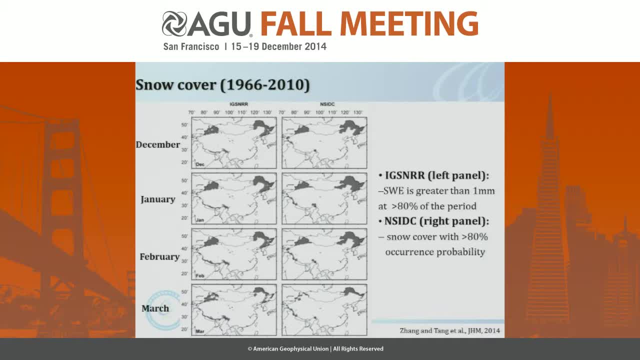 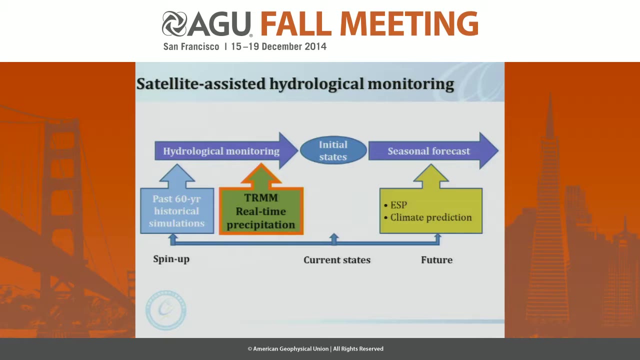 We compare the model- similarly- the slow curve- with the satellite-based model, The model can produce the slow curve. well, We get a long-term hydrological simulation. I think it can capture the hydroflux on the stage in China. Based on this long-term data set, we are going to do the hydrocommoniting. 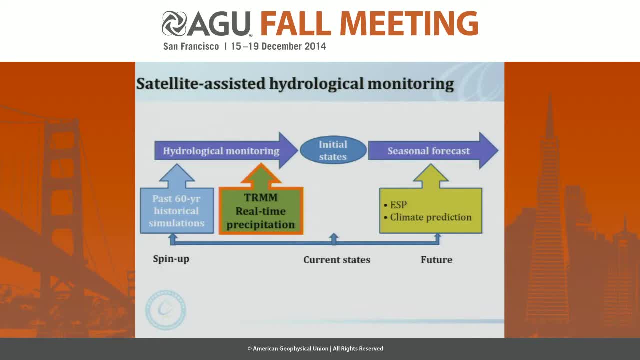 In that case we need the new real-time forcing. Now we are not able to gather the new real-time observations. We don't have precipitation observation from ground stations yet, so we decided to use the satellite to train real-time precipitation and input the model. 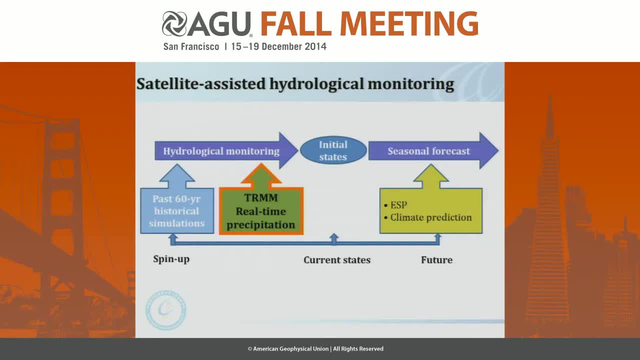 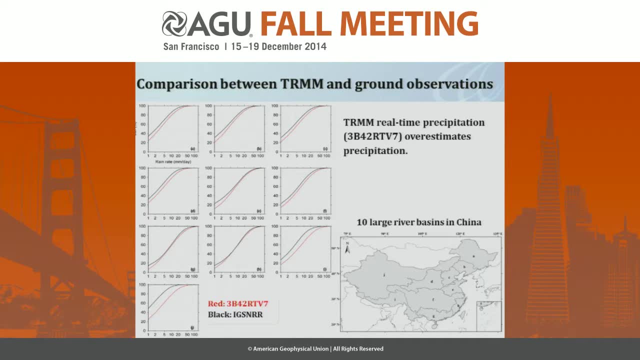 The issue is how to make them consistent. This slide shows the comparison between the satellite and the ground observation. So actually the data is not consistent, So the treatment data always always made precipitation. The water is a large layer basin in China. 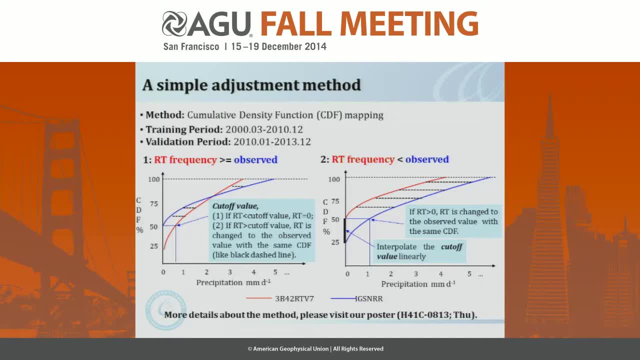 That means we are not able to directly compare the new real-time estimates to the historic estimates, so we use a simple adjustment method called CDF mapping. The basic idea is: in the training period we found the difference between these two data sets and find the relationship. 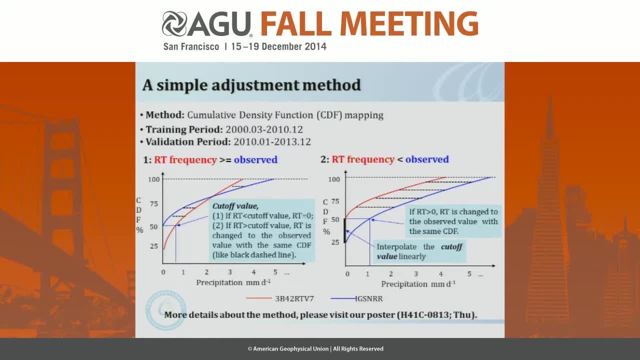 And then we use the data, this relationship, to adjust the real-time precipitation. I'm not going to go into detail about this method. For more detail, please visit our poster, which will be presented tomorrow. So this shows the performance of this adjustment. 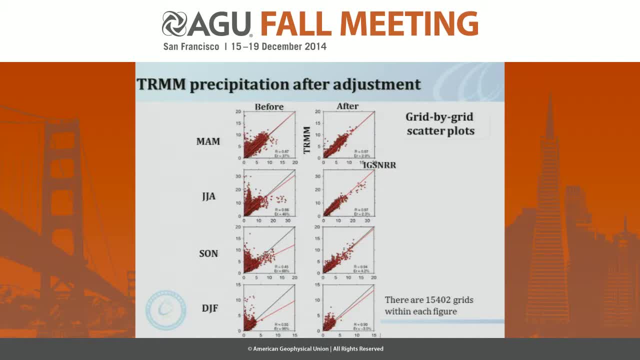 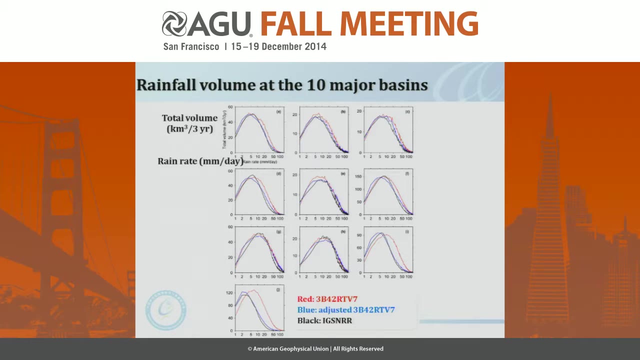 Before adjustment: there are a large difference between the ground-based and the satellite estimate. After adjustment, all the grays goes to the one-to-one line And we also compared the total rainfall volume at the 10-notched-ray basin. So before adjustment, if we use the satellite data, 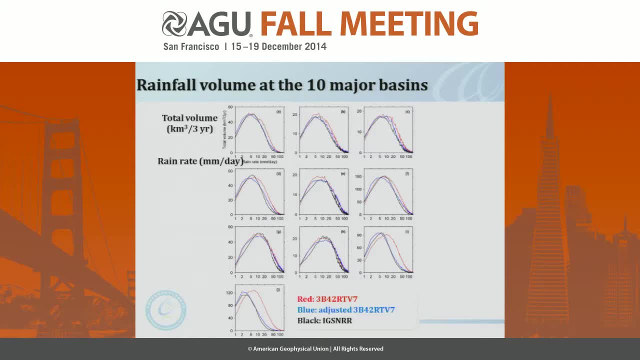 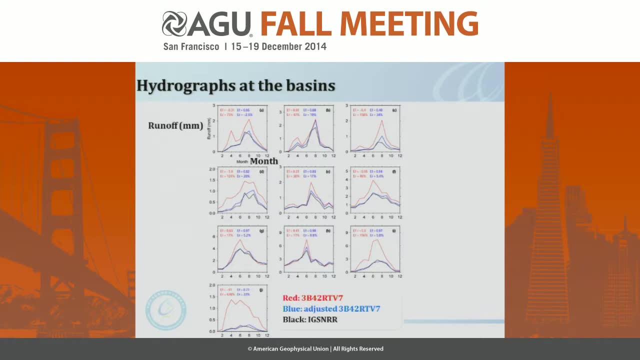 it will always make the rainfall, but after adjustment it will agree with the observation-based estimate. We compared the hydrograph at the basin to the high-flow at the basin, Of course before adjustment, if we would directly use the satellite data. 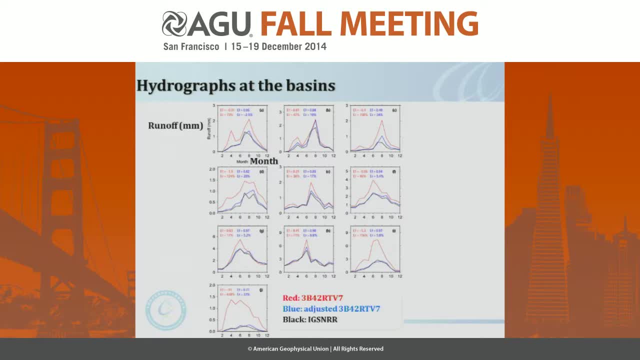 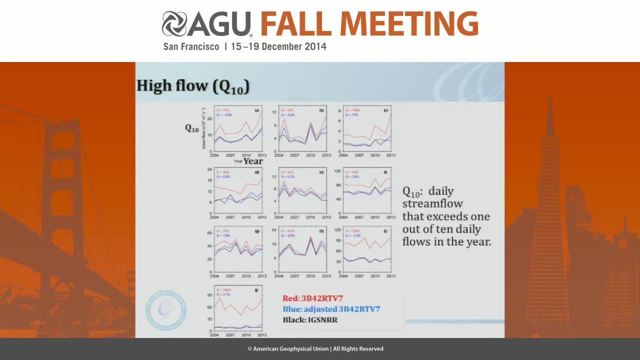 actually we would get much higher stream flow. that would cause much more force over flooding risk. So after adjustment it would agree much better with the observations For the high-flow in flooding season. usually it's the same if we use the satellite data.